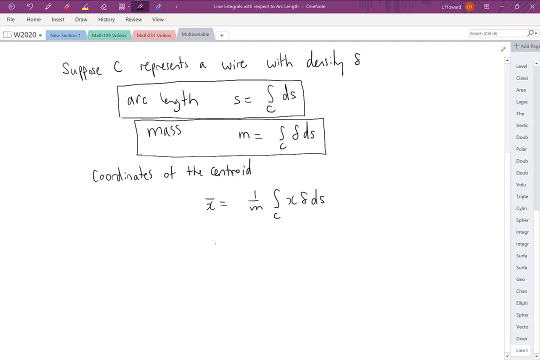 along our curve of x delta ds. And similarly we could get y bar and z bar. So let's look at some of these formulas. So for z bar, for example, we'd take 1 over our mass times, the integral along our curve of z delta ds. We can also talk about the moments of inertia with respect to the 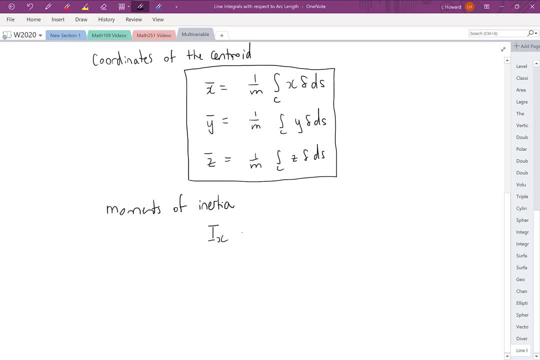 three axes. So if we want the moment of inertia with respect to the x-axis, we would take the integral along our curve C of y squared plus z squared, delta ds, And similarly we could look at the other two moments of inertia with respect to the other two axes, And similarly we could. 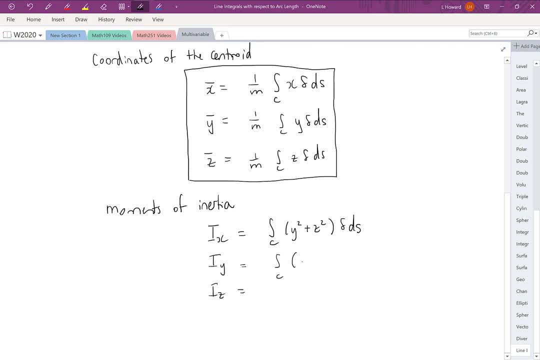 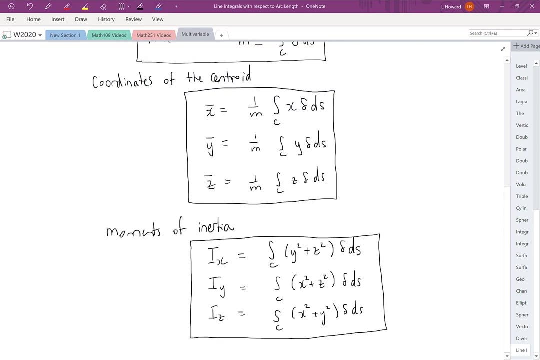 So in each case our integrand is going to be the sum of the squares of the other two variables. So for y sub y, integrand would be x squared plus z squared delta ds. So there we have our formulas for our moments of inertia, our centroid mass and arc length for a wire with a given density. 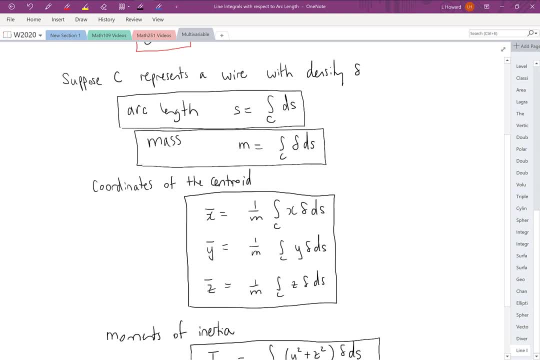 These integrands are the same as the integrands that we used for a double hardly time in any sense curve, So we can also use them to talk about the moments of inertia and triple integral, And similarly we could look at the thermal density تو delta ds. or the Sheila integral for the order stock of the 머�. любой scale measure. What we'd integrate would be z star minus the length. This was going to be 1 over g square delta ds. So as we've taught, we could take this interval. we can identify it byenter mouse range. 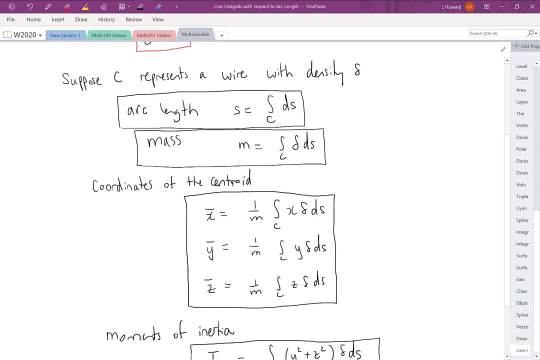 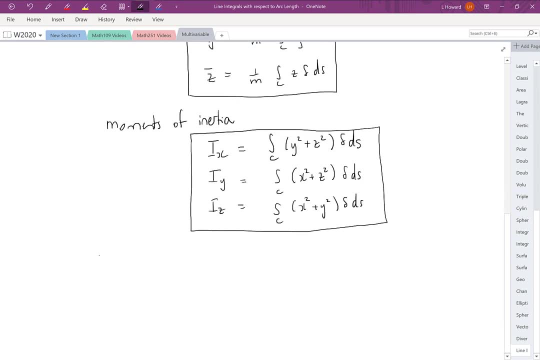 integration earlier in this video series. So we're now just applying them in a slightly different physical context, where we've got a wire with known density In order to get into a calculation. what we need is a formula for how we're actually going to calculate ds. So there, 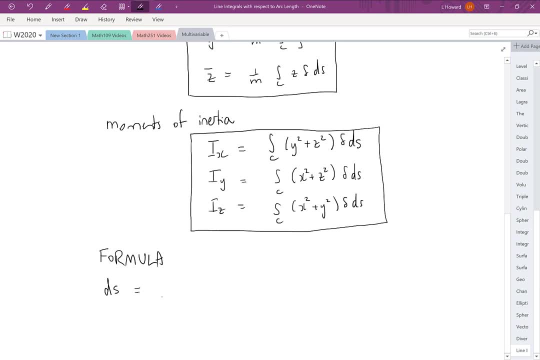 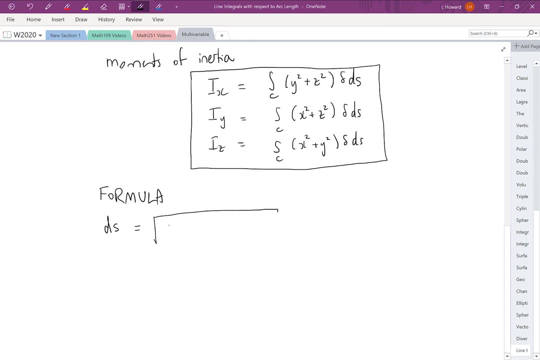 are going to be two variations here, depending whether we're in 2d or 3d, So we'll write down both variations. If we're in 2d, then ds is going to be the square root of dx by dt squared, plus dy by dt squared, and then outside the root. here we're multiplying by dt, So that's. 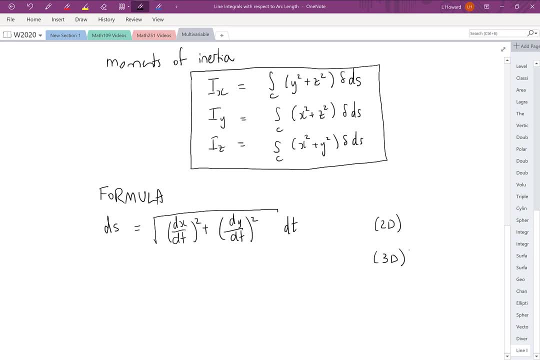 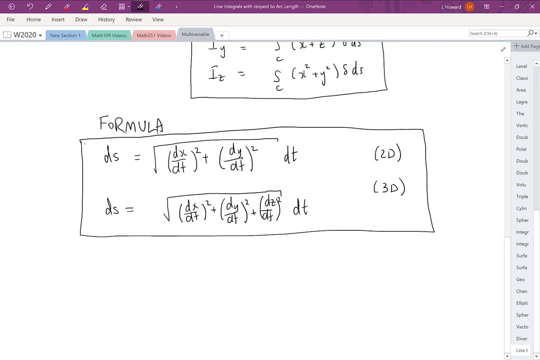 the 2d version and a 3d version quite similar. It's just got an extra term under the root, corresponding to the z variable. Before we jump into an example, let's draw a quick picture and try to understand where this formula for ds comes from. I think this will be most clear if we just 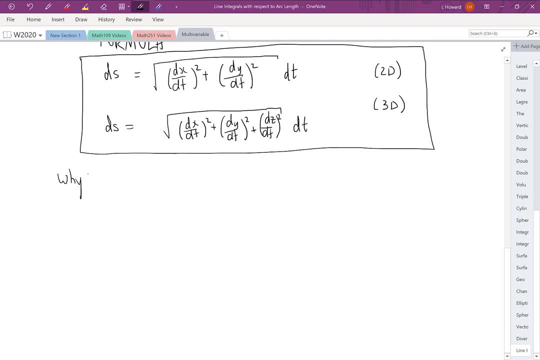 look at the 2d example. So let's just ask: why is this formula true? looking at the 2d formula, Well, imagine that we've got a curve c and what ds represents is just a tiny, infinitely small chunk of the arc length along c. 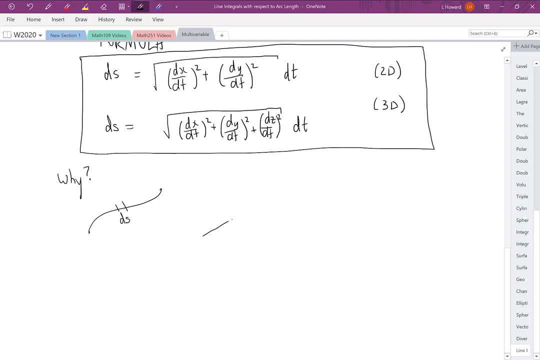 So if we actually zoom in on ds, we could say, over a very tiny interval ds is basically a straight line segment. So let's say that's ds there and that ds is a straight line segment. So let's say that's what we're going to do. Let's say that ds includes a little bit of change in the x direction. 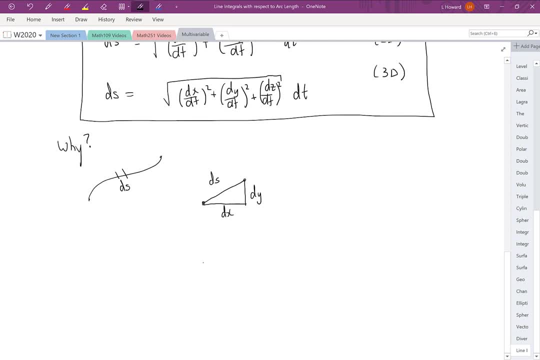 and a little bit of change in the y direction, which we'll call dx and dy, So by the pythagorean theorem, because we could say ds is going to be the square root of dx squared plus dy squared. So we could take this quantity and we could multiply it by dt over dt, And let's take that factor of dt. 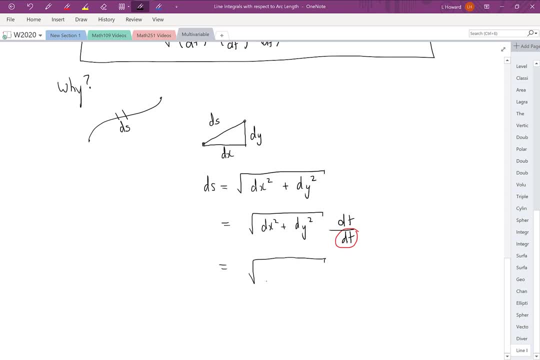 that we're seeing in the denominator and let's bring that inside the square root. So when we bring that inside the square root, then the deno m a is also the square root of the square root of ds, square root That's now going to become a dt squared in our denominators. So under the root, 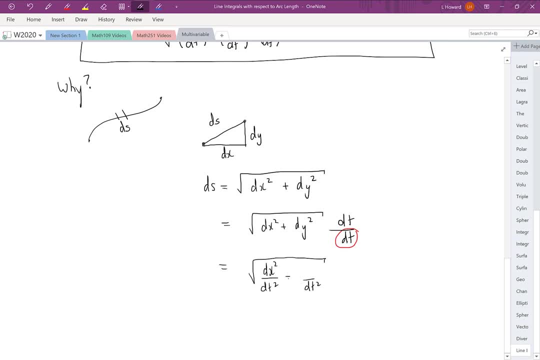 we're going to have dx squared over dt squared, plus dy squared over dt squared, and then we still got that factor of dt out at the back. So with a little bit of bracketing, that's going to look like the formula that we wrote down above, So we could say under the root, we've got dx by dt. 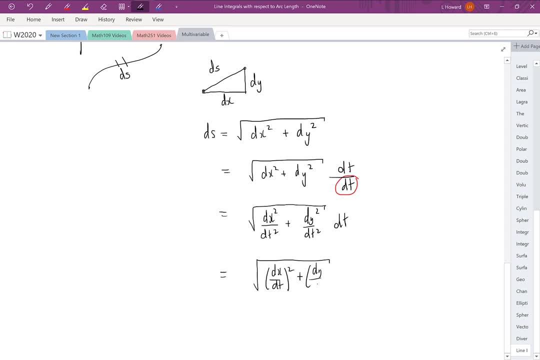 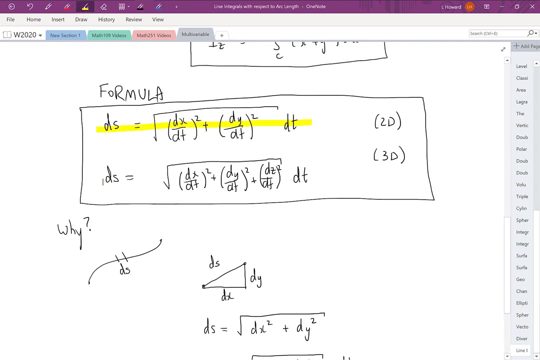 squared plus dy by dt squared and then that's times dt. So that all goes towards justifying these formulas for ds that we wrote up a little bit earlier here, and these formulas are what we're going to need if we actually want to do a computation for a line integral, with respect. 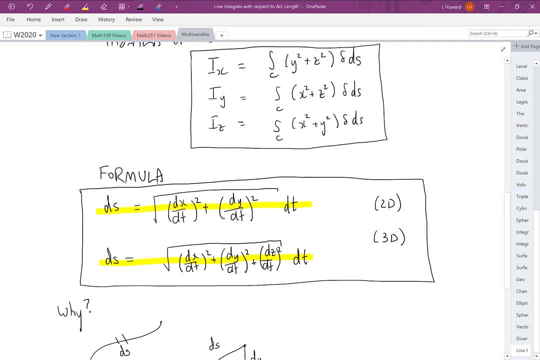 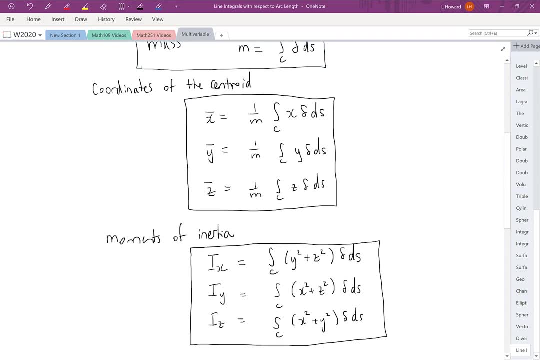 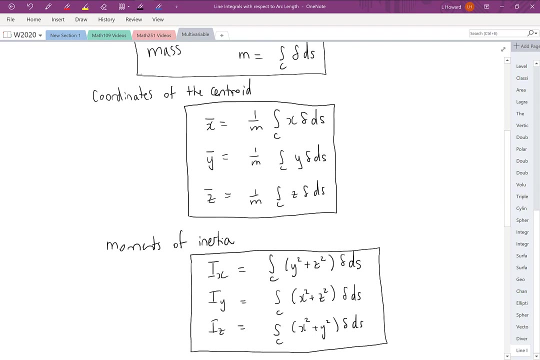 to arc length. So we mentioned at the beginning of this video that we're going to be computing integrals of the form, integral over sum, Curve of sum, function times, ds. So all these types of integrals that we've written down here and these types of integrals where we're integrating along a curve are called line. 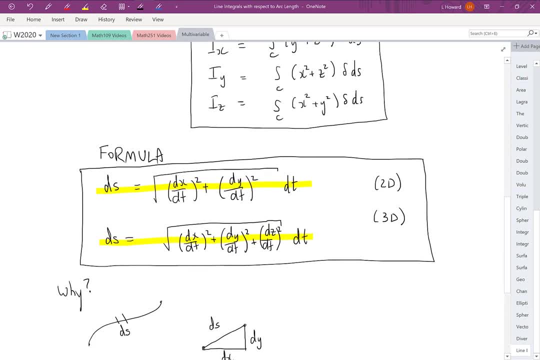 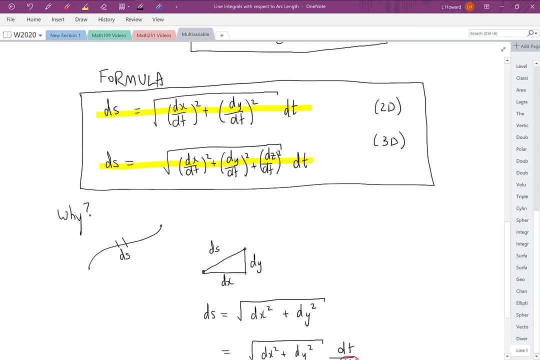 integrals. Despite the fact that our curve may not be a straight line, we still call the integral line integral. I suppose curve integral might be a better name or a better way of thinking about it, but line integral is just the historical name for this type of integral. So anytime we see 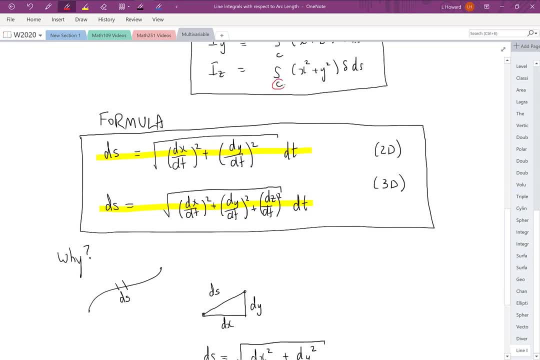 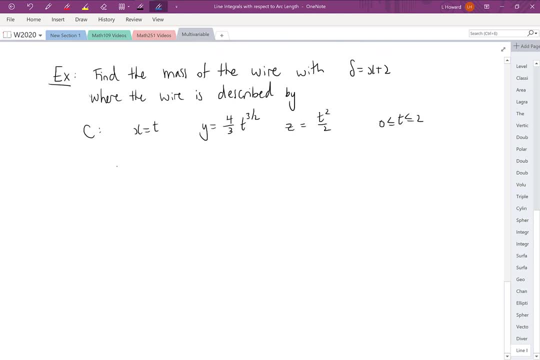 these integrals where we say we're integrating along c. just picture a curve could be in 2d or 3d. So here's an example of how we compute a line integral with respect to arc length. What we want to do in this example is find the mass of the wire with given density function where the wire is. 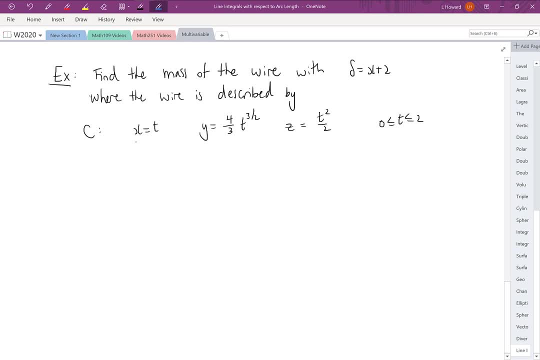 described by the following curve. So we've got this curve in 3d. we're describing how the x, y and z coordinates change as the t values range from 0 to 2.. So basically, at t equals 0, we're mapping out some point in space. at t equal 2, we're mapping out some other point and then, as those t values vary, 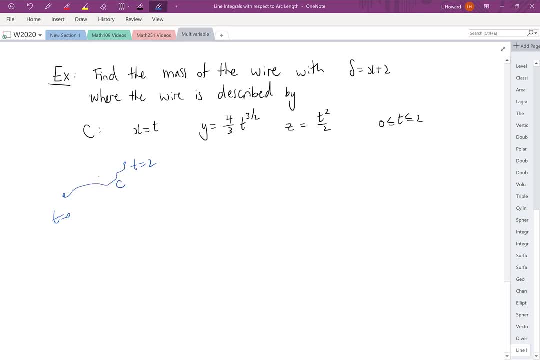 our curve is moving in some way through three-dimensional space, So the first thing we're going to work towards here is coming up with a formula for ds. We're going to need that in order to set up the integral for the mass of the wire. 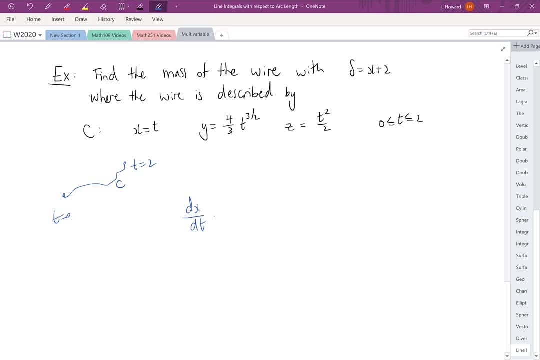 So we're taking the derivatives of our different x, y and z variables here, taking our derivatives with respect to t. So dx by dt is going to be 1, dy by dt. well, we would have four thirds times three halves t to the one half. so let's just call that 2t to the one half and dz by dt is going to be t. 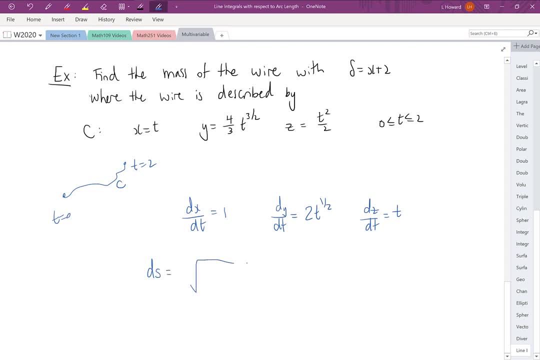 So with that we can break out our formula for ds. So, as we said above, we're going to be taking the derivative. ds is going to be a certain square root times dt under the square root. we're going to have the sum of the squares of these different derivatives, So the dx by dt squared plus the dy. 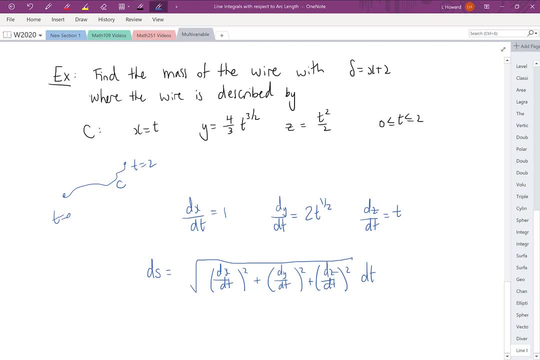 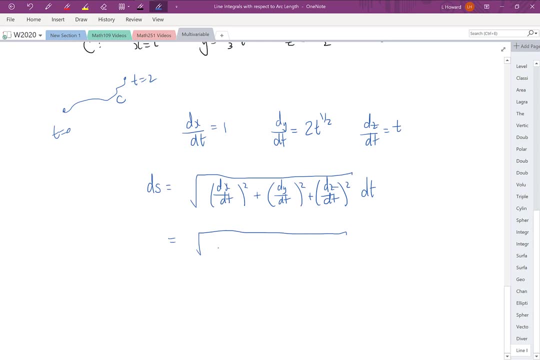 by dt squared plus the dz by dt squared. So let's sub everything in here and get a nicer formula for our ds. So just squaring each of our derivatives and summing up, we're going to have 1 plus the square of dy by dt is going to be 4t. 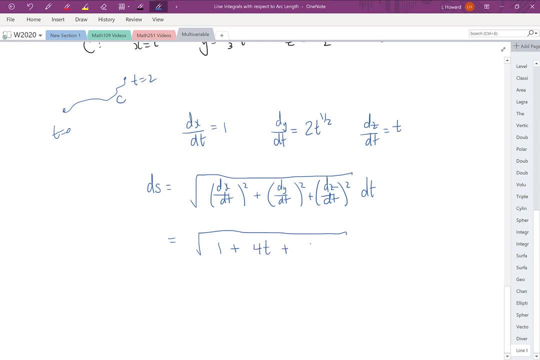 And then plus the square of dz by dt, that's going to be t squared and that's all times dt. So now we can say mass is going to be the integral along our curve of delta ds. So in other words, integrating along our curve, we're told in the question. 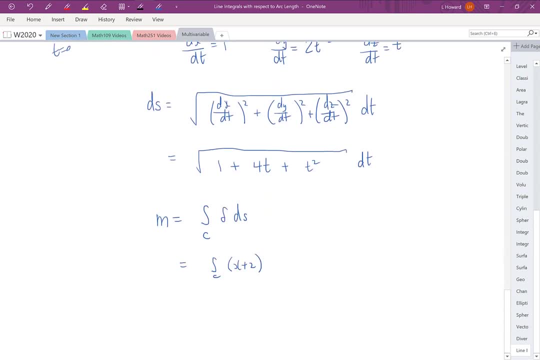 that our density function was x plus 2, so we'll just sub that in there and then that's times ds. So in order to turn this into an integral that we can calculate, the idea is to move everything over into the variable t. So there are three things we want to transform over to t. we want: 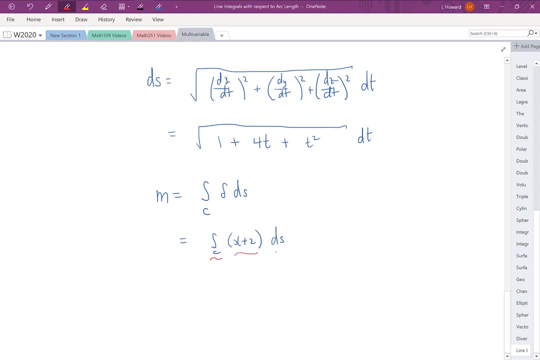 to change the limits of integration over to t. we want to change our integrand and also our ds. So here's where our formula for ds above comes into play. we'll be able to just substitute in there to get ds in terms of t, To get the x plus 2 in terms of t. we can look back to our problem. 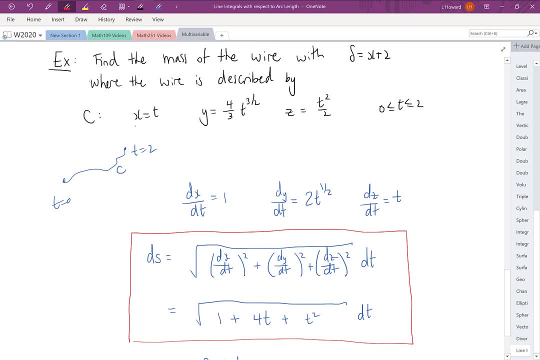 remember we were given formulas for how x, y and z depend on t. So we can just replace our integrand with the appropriate functions in terms of t and then to get our limits of integration again, those would be given as part of the problem. t would be ranging between 0 and 2.. So I think we're ready. 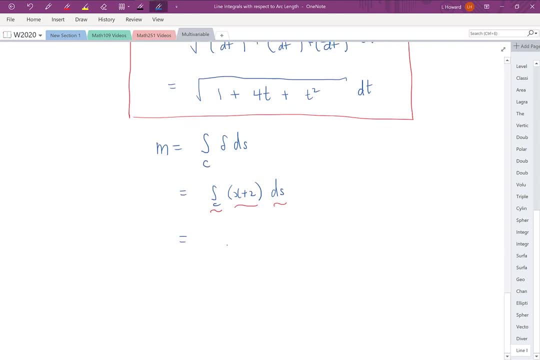 to plug everything in and get this switched over to the variable t. So we said t is going to be ranging from 0 to 2.. We were told that for this specific wire or this specific curve, x is equal to t, so our integrand becomes t plus 2. 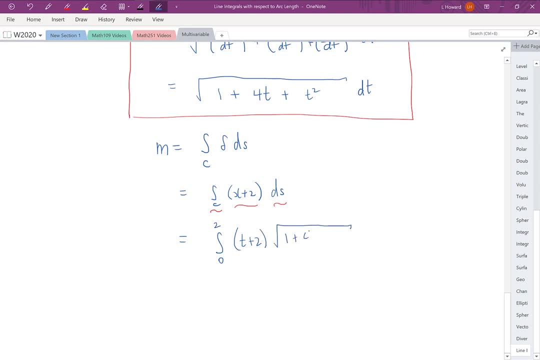 and then our ds is the square root: 1 plus 4t plus t, squared times dt. So we've now got an integral entirely phrased in terms of t and we're ready to proceed with the integration. So let's try a substitution here to get this done. let's sub u equal the quantity under the root. 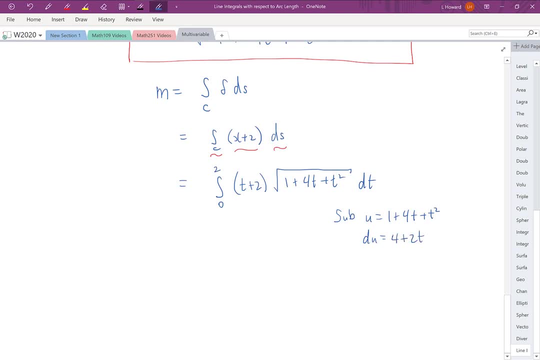 That would make it 2 minus 4t, so it would end up being t. So now we can just quote this from the end of the equation: make du equal to 4 plus 2t times dt, and that means that du over 2 is equal to 2 plus t. 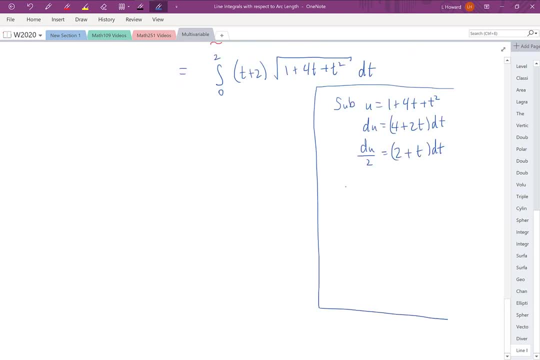 times dt. So for the sake of our substitution, let's say we're trying to compute the indefinite integral of t plus 2 times this root times dt, and we're going to say: well, that's the same thing as integrating root u and then the t plus 2 times the dt we said is: 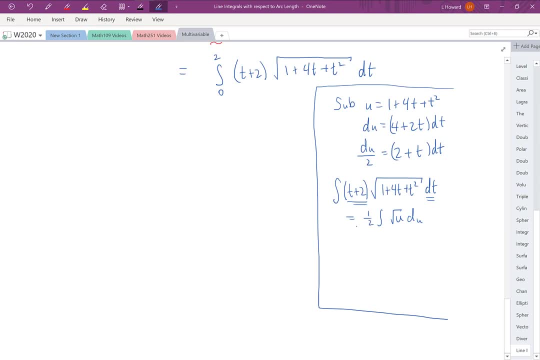 the same thing as du over 2.. So let's write this as 1 half the integral of root u, du, and then we can say: well, integrating the root u, we're going to have u to the 3 halves times 2 thirds, and we can say: plus: 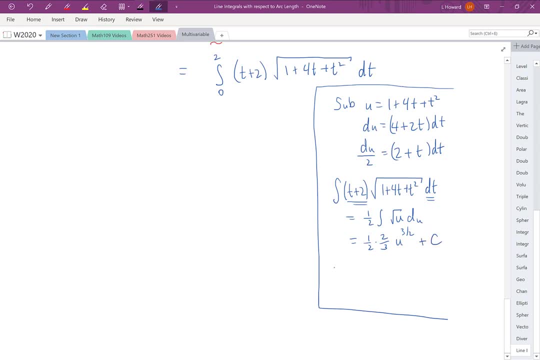 c, just because that's good form with indefinite integrals, and then we can write down our answer. So that would be 1 third Times something to the power 3 halves, where the something is our u, so the 1 plus 4t plus. 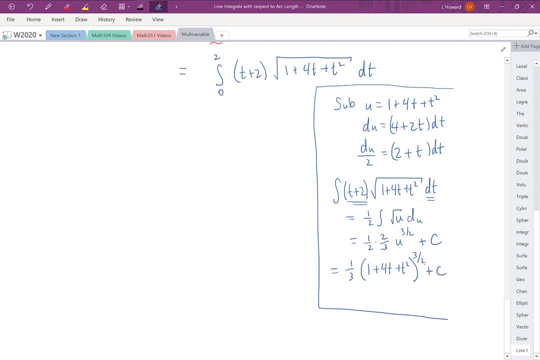 t squared, and then we'd have our plus c on here just for good measure. So with that we're ready to finish off our integration, and I think I'll just write our final answer up here just below our integral. So our integration gives us 1 third, 1 plus 4t, plus t squared to the power, 3 halves and 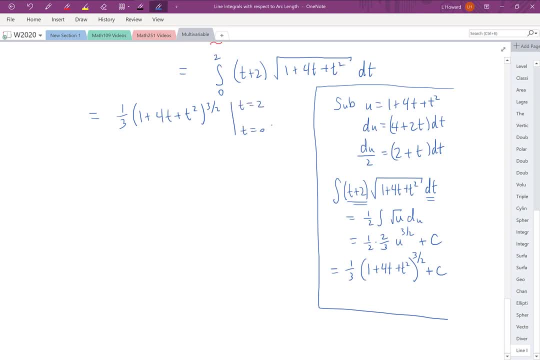 we're going to evaluate that at t equal 2.. And then t equals 0. Well, both of our expressions are going to have the 1 third on there, so we might as well factor that out And then, subbing in t equal 2, we'd have 13 to the 3 halves, and then subtracting off. 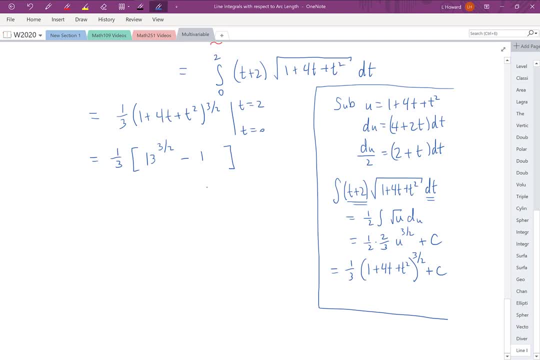 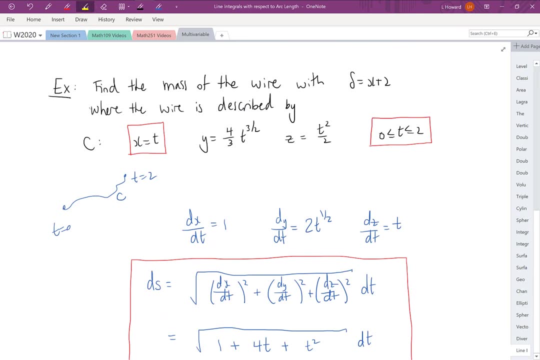 our value at t equal 0,, we'd have 1.. So what that's giving us is the mass of the wire, with given density function, where the wire has a prescribed shape. So we were told what the points x, y and z were along that curve. 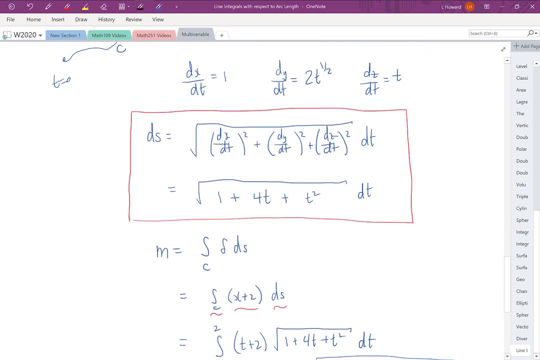 And the way that we actually computed the mass of that wire was by setting up this line integral, Line integral just being a fancy way of saying, hey, we're integrating along all the different points along some curve, And you can do that in either 2D or 3D.